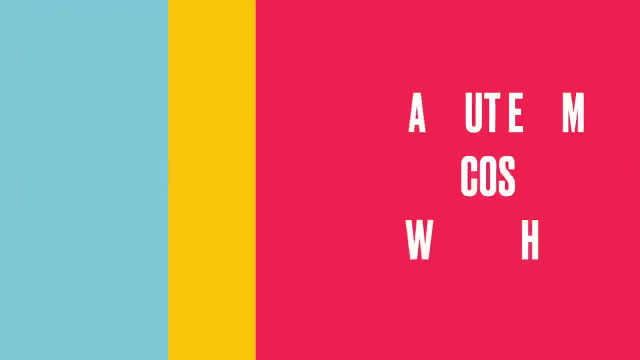 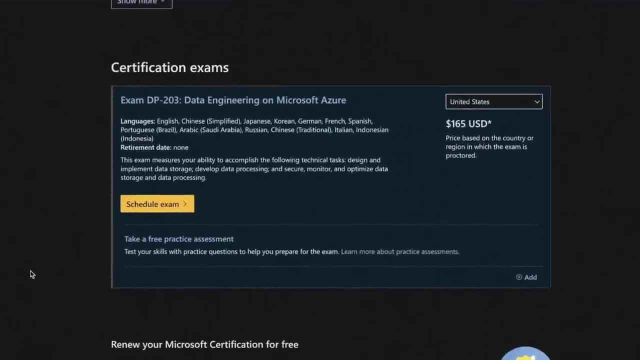 taking notes if you want to remember it better. So we will start this video by understanding the basics about the exam, the cost of it and how to schedule it. So DP203 is an Azure Data Engineering exam that validates your knowledge in designing and implementing data storage. solutions So you can clear this exam within 20 days if you use the framework that I will give in this video. I will highly suggest you to watch this video from start to end so that you don't miss out on any important information. So you can grab a pen and paper and start taking notes. 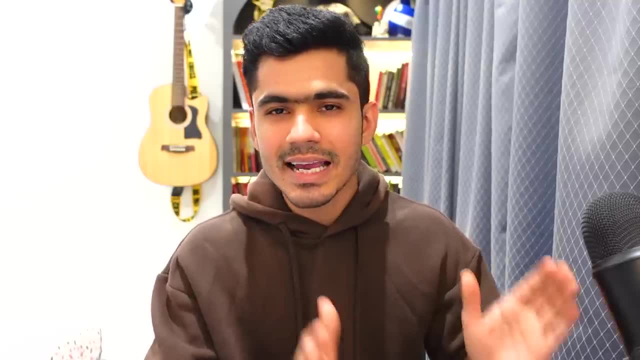 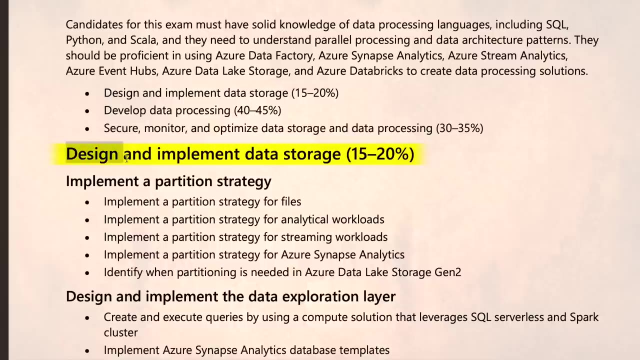 using Azure Cloud technology. Basically, you should be able to design and solve any data engineering problem using Azure Cloud technologies. The exam will test you on these three sections: design and implement data storage. 50 to 20% of the topic will come from this. You should know. 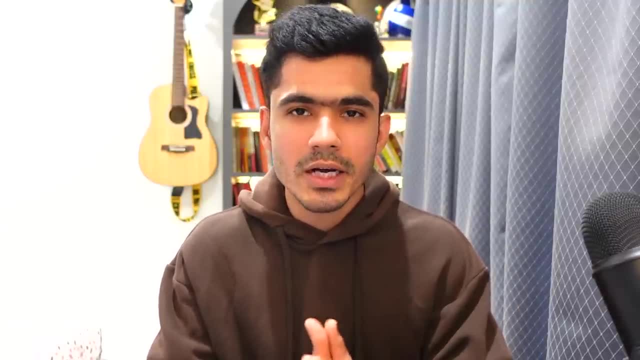 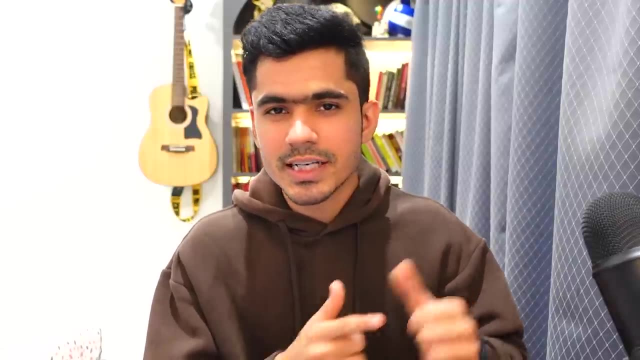 how to properly store data using different storage services provided by Azure. Developed data processing. 40 to 45% of the exam will focus on this. There are many different services provided by Azure, such as Databricks, Synapse, Analytics, Azure Data Factory. All of these services are used. 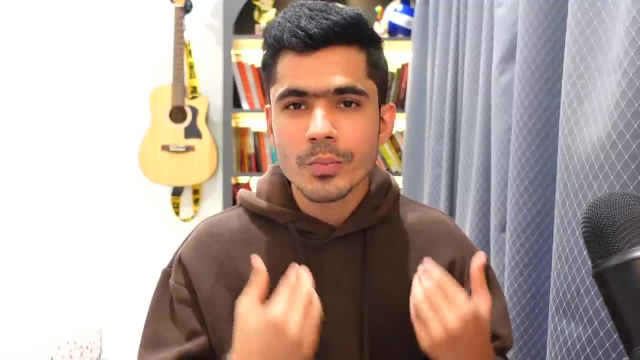 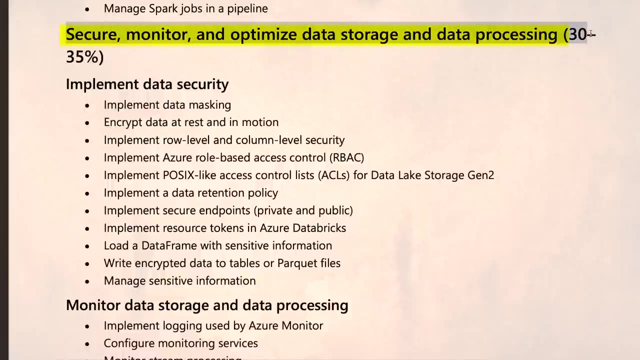 for data storage, processing and analytics. So you should know how to properly process your data using different services provided by Azure: Secure, monitor and optimize data storage and data processing. 30 to 35% of the exam will cover this. Security is one of the main concerns. 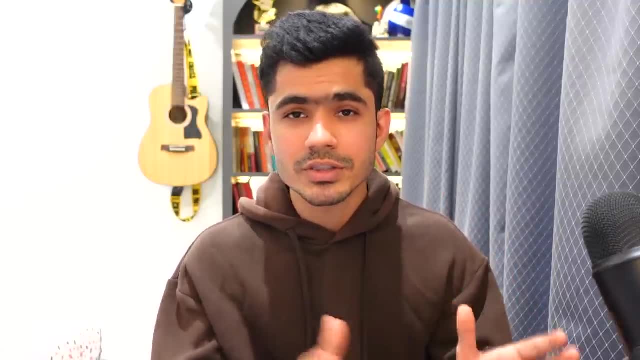 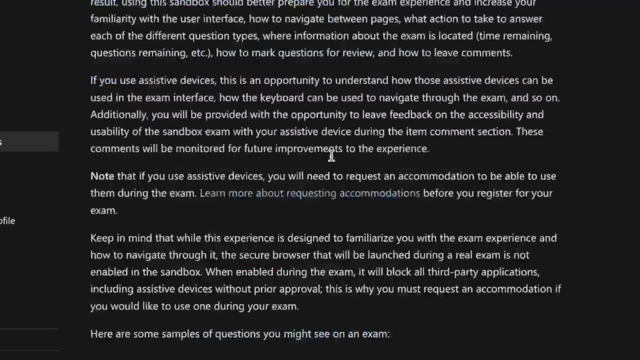 of any company And, as a data engineer, you should know how to securely process all of these data. The length of this exam is around 120 minutes and you will have 40 questions in front of you. that will contain different types of questions, such as case studies, multi-answer and single-answer. 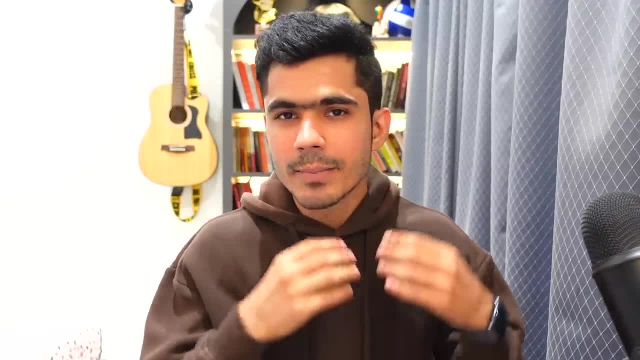 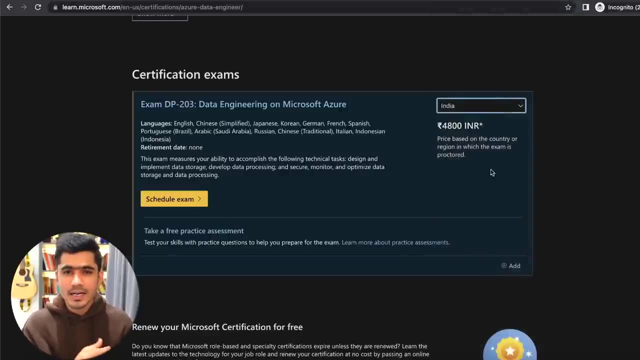 questions. Top 10 questions will be answered. Top 10 questions will be answered. Top 10 questions will be answered. The cost of this exam depends on the country you live in. So if you live in US, it will be around 165 USD. If you live in India it is around 4,800 rupees with some taxes. So 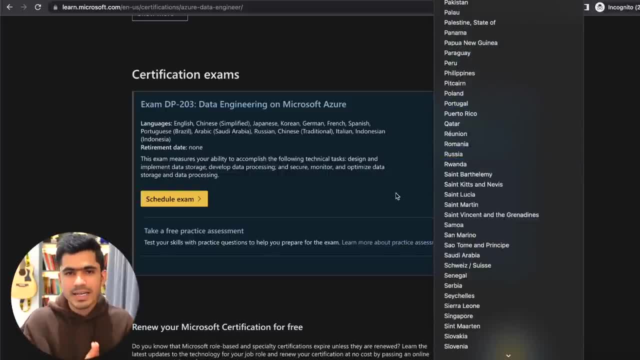 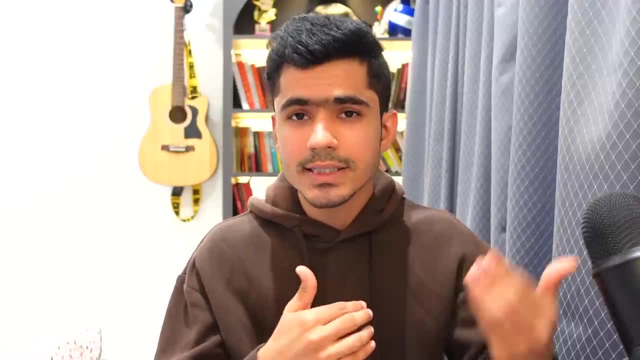 it changes country to country, So you can just go to this certification website and check and understand about that. If you want to appear for this exam, then you can just click on this button. There are two different options. One is you can go to the test center and appear for this exam. 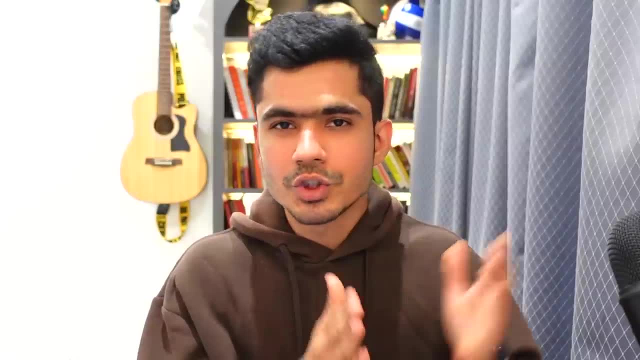 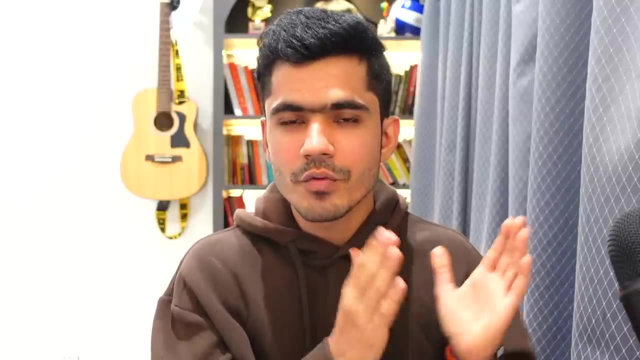 Or, if you want, you can give this exam from home, But, depending on your comfort, you can choose any of the options, fill the form, pay the money and schedule. Now. you don't really need to have any prior certification experience if you want to appear. 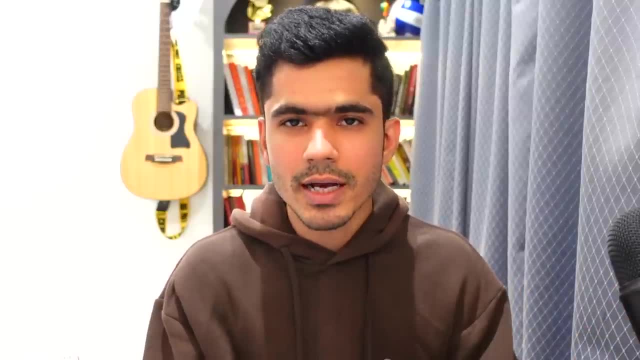 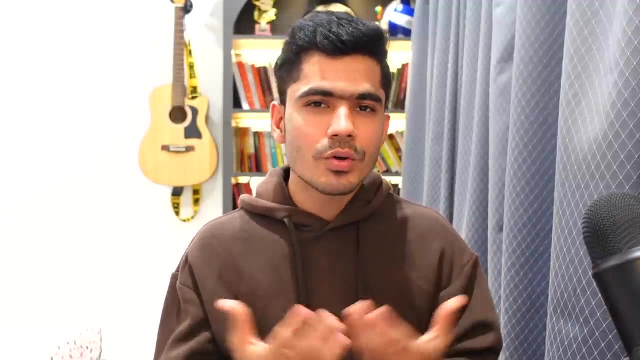 for this exam. Before this, I had no understanding about Azure and this was my first certification, But it is recommended that you know the basics about Python, SQL and basics of data engineering. If you want to learn that, I already have some of the courses available on my website. So 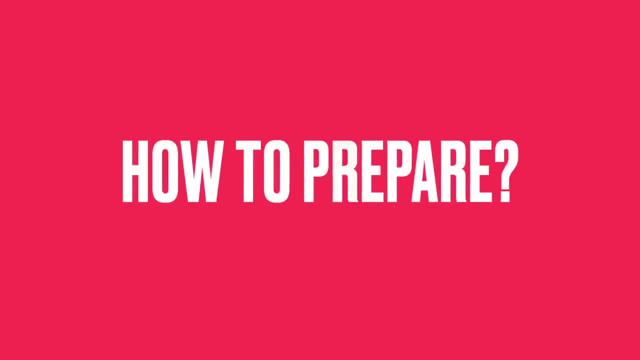 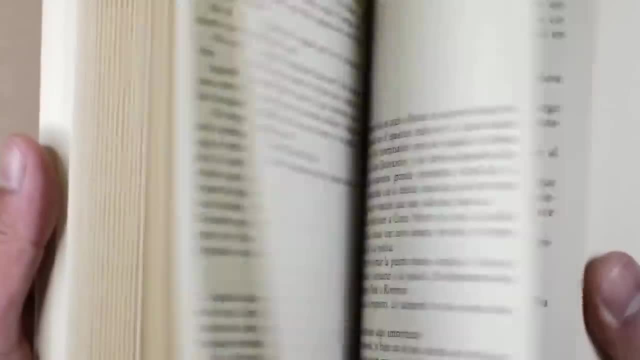 you can go and check it out Now. this was all about the exam. Now let's understand how to properly prepare for it. The first step here is not to master anything. It is just to capture the information that is coming at you. 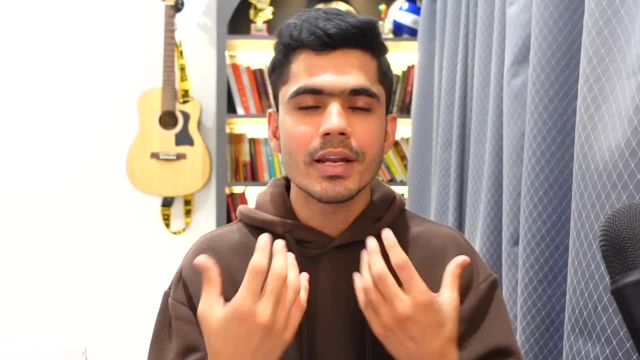 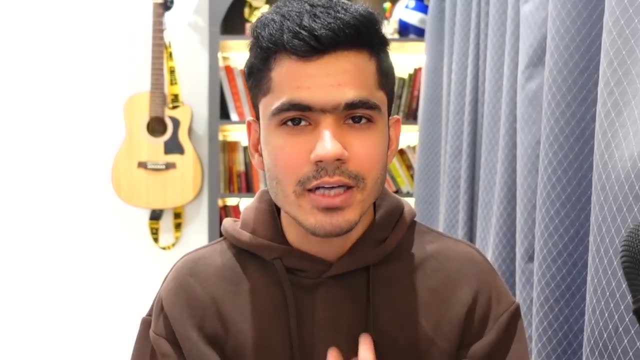 Most of the people, when they start learning about any certification or any cloud platform, they tend to give up at the initial phase only. The reason is they can't handle the information that is coming to them. It is too much, and they think I won't be able to do any of these things. 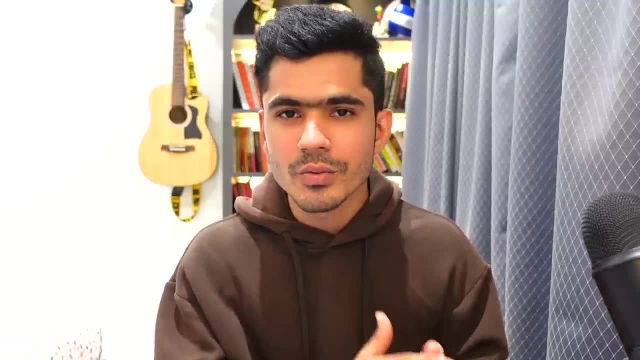 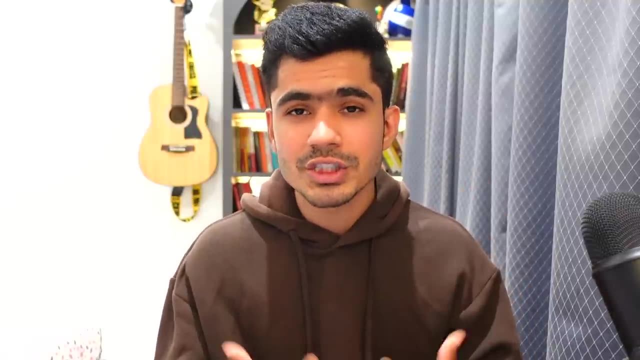 First step is the hardest and most of the people give up here only Because when you start learning any new thing- it can be cloud platform or preparing for the certification- there are so many new information that is coming at you. People think that they need to master all of these things. 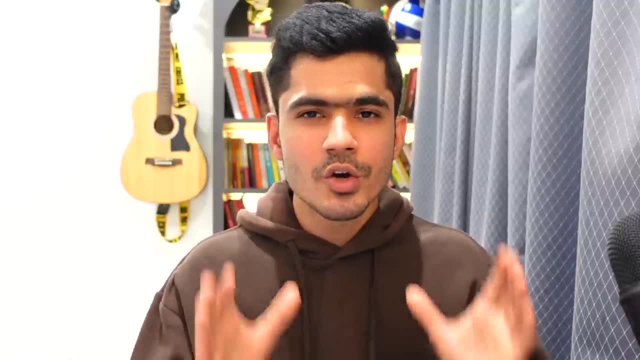 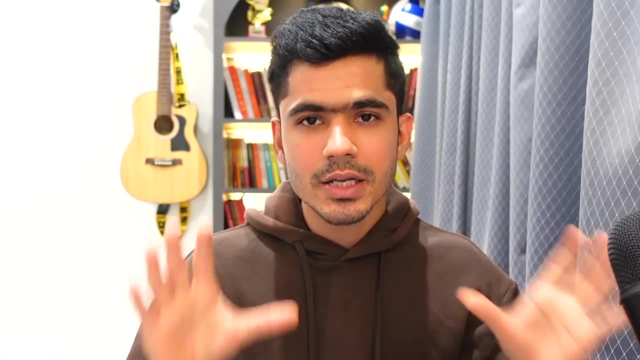 by watching one video. This is not how things work in the real world. When you are starting to learn anything, all you need to do at the initial stage is to get familiar with the different terminologies and components attached to that particular thing. So in this case, we are preparing for Azure cloud certification. The first step here is not 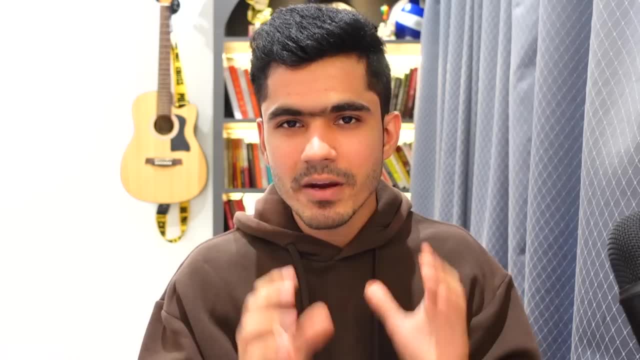 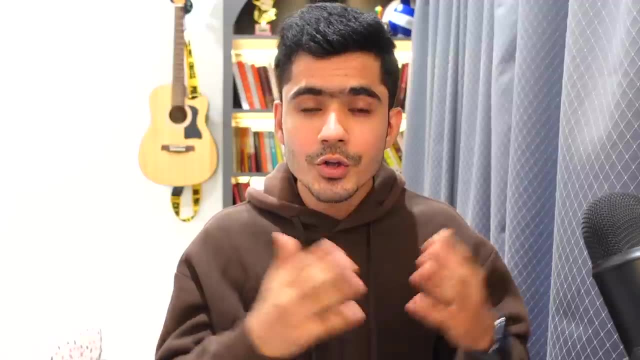 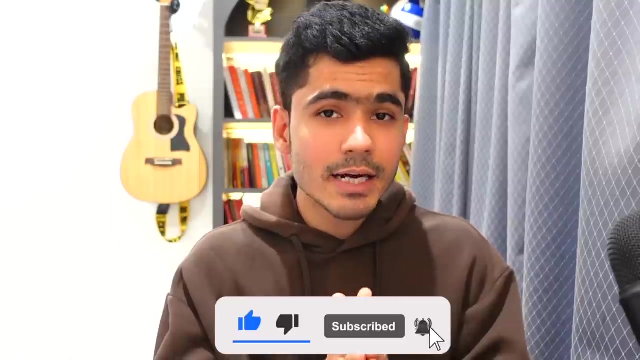 to master everything about Azure cloud is to just get familiar with the different services and components attached to it. Before this exam, I have never opened Azure cloud portal or knew about any of the services they provide, So it is really important that you get comfortable with the ui and different services provided by azure. again, it can be. 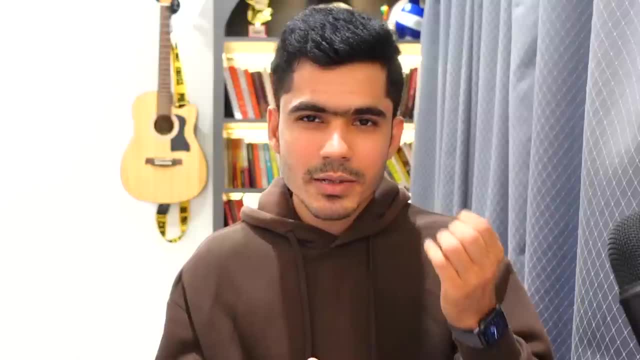 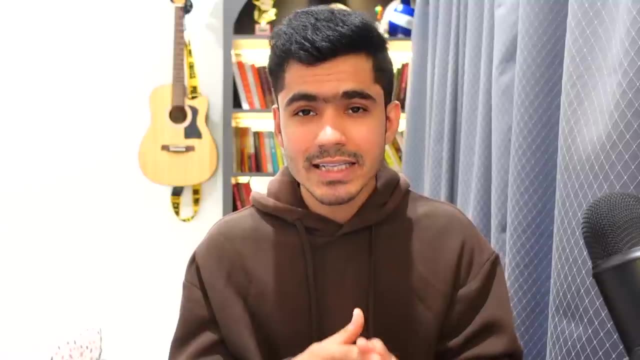 difficult when you are just starting to learn any new thing. there is a little bit discomfort when you're trying to understand the new information, but you don't have to give up at this stage. you don't have to master anything like this. you just need to let the information flow to you and it's 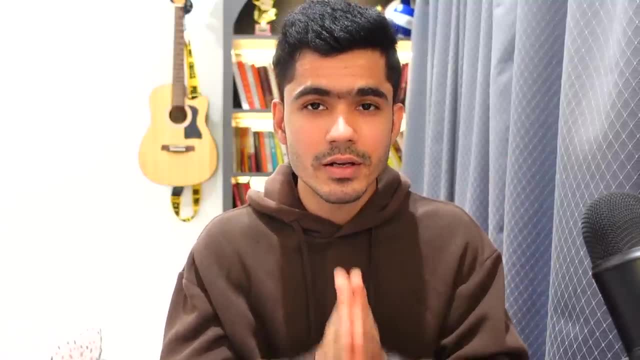 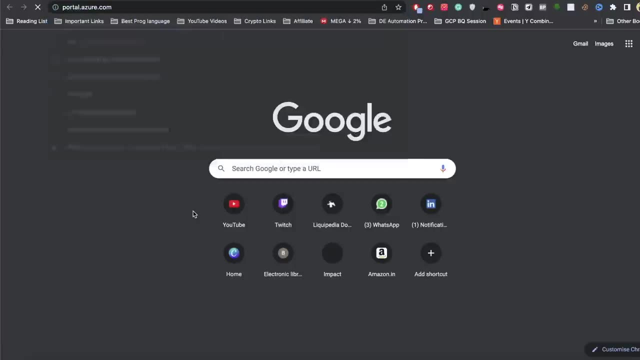 okay, even if you just understand five percent of the things that you are learning. so there are two things that i did. first, i created my account onto azure cloud. you can just go to the portalazurecom create your account for free. they give you the 12 months free trial and 200 usd to practice. so you 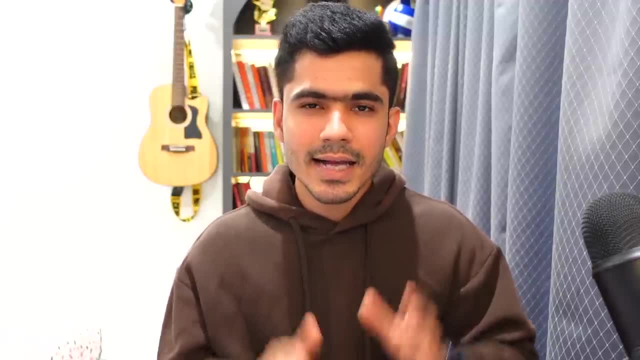 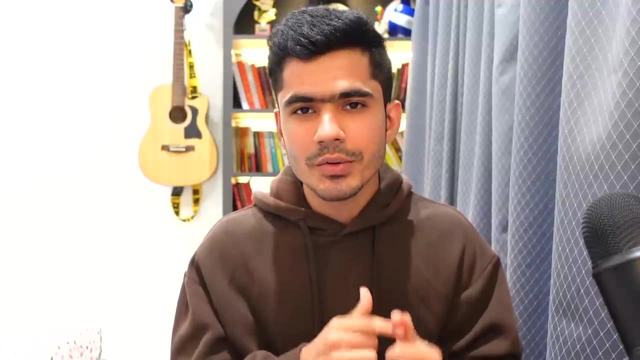 can just go to the portalazurecom and create your account for free, and then i spend around one hour just exploring the different ui and the services available on azure cloud. with this you can also start doing the free training provided by microsoft itself. it is available on this website. 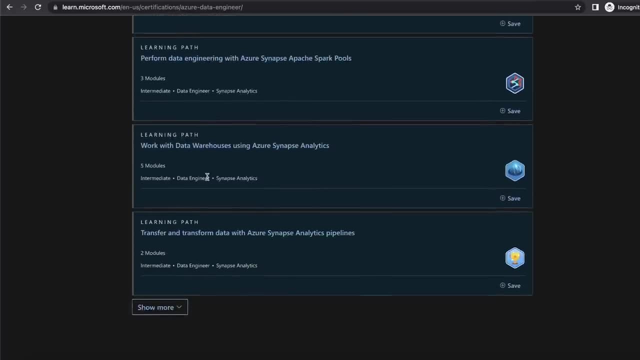 and it is completely free. the way to learn is that you can go through this training and whenever they mention any service name, such as azure data lake, you can go to azure portal, search about the services and get free training on azure cloud. and then you can go to the portalazurecom and you can. 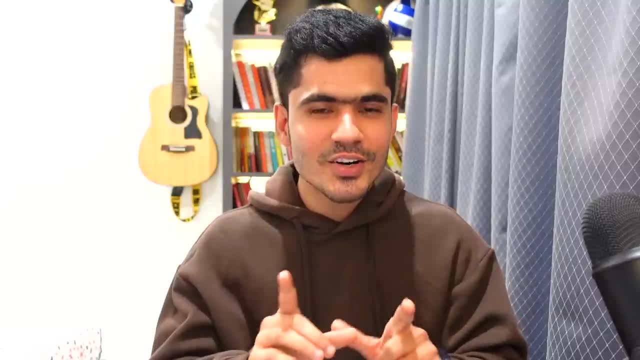 go to the portalazurecom and get free training on azure cloud. and then you can go to the portalazurecom familiar with the ui and different options provided by them. again, we are not doing this to master anything. all you need to do is get familiar with different components and services provided by. 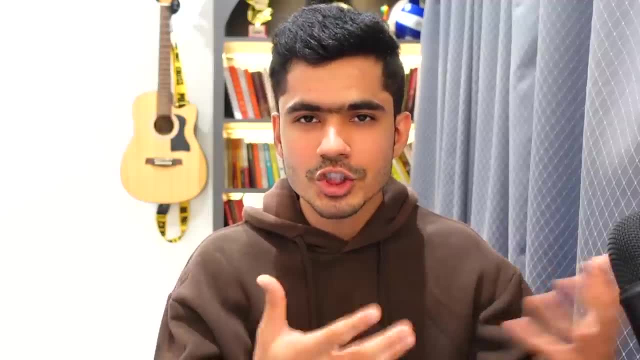 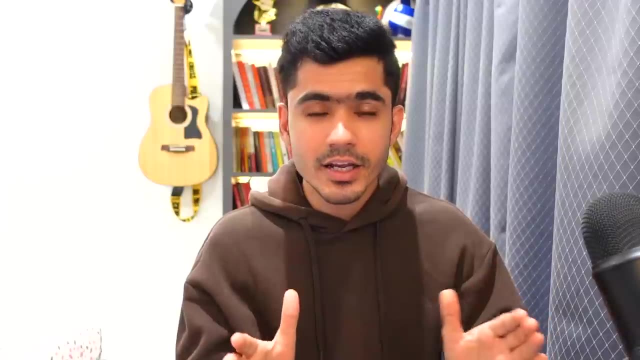 azure and get comfortable with the ui, such as understanding about the azure data lake service. it is used for building a data lake. you should be able to summarize the entire thing in just one line when you go through this training again. you don't have to master everything, you just need to. 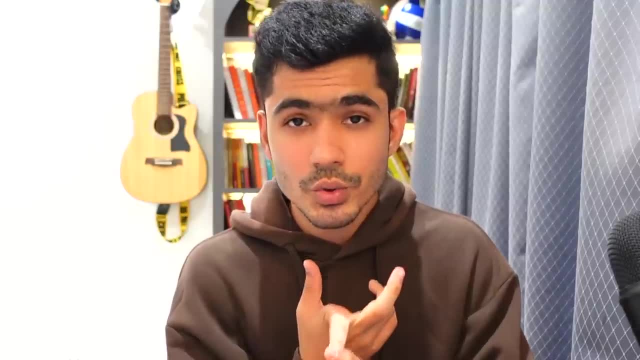 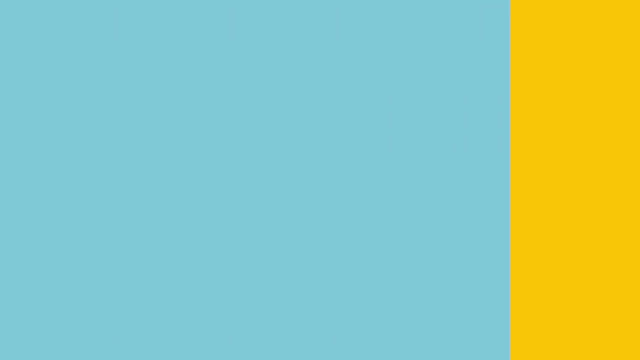 have the basic understanding of what it does. so in this step we focused on two things: one is getting familiar with the ui and second, having the basic understanding about the data lake and the services, all of these different services. once you have the basic understanding of it, then we can go and deep. 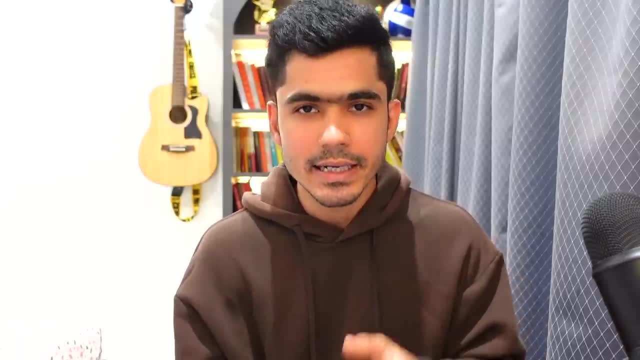 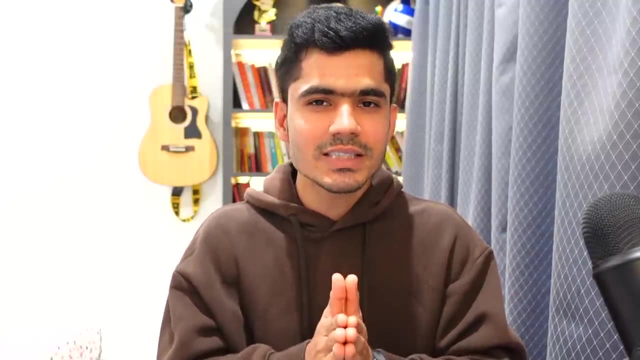 dive into individual topic and understand it in detail. now there are two resources that i use in this section. one is course and second one is book. i did both of these things simultaneously, so the first thing that i use is the course content. now it doesn't really matter which course you choose. 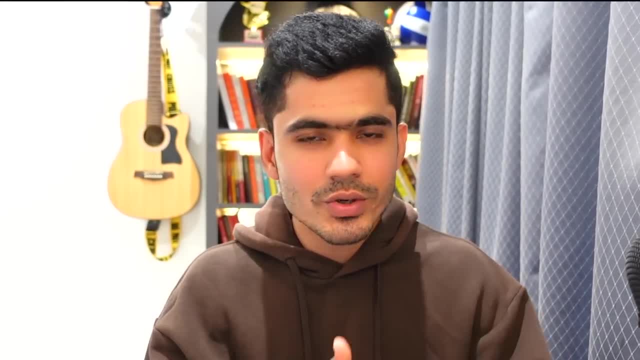 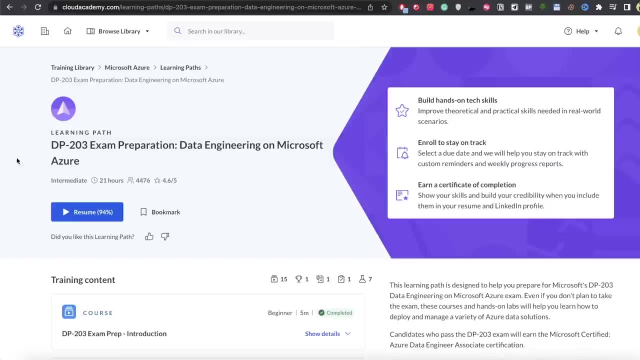 but i will recommend you a few courses because a lot of my audience is students and freshers and they want affordable courses. so i will recommend you a few courses so you can choose one from that and start learning about azure cloud. the course that i used was from cloud academy, dp203- azure data engineering associate. this course will teach 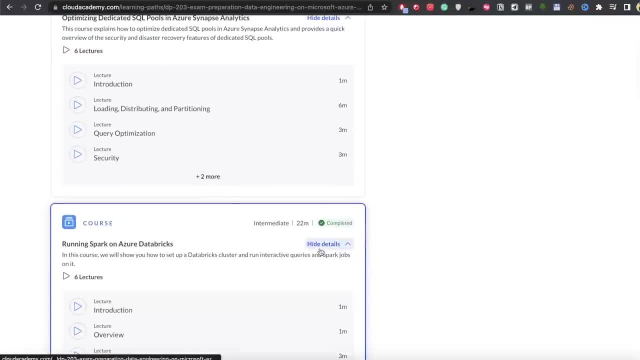 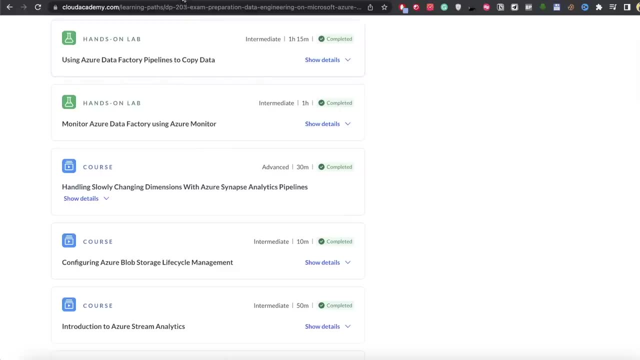 you everything you need to know about azure data engineering services and basics of data engineering. plus, they come with the hands-on lab so you can also build mini projects. alternative for this course is also available on coursera: microsoft azure data engineering- associate dp203- this course. 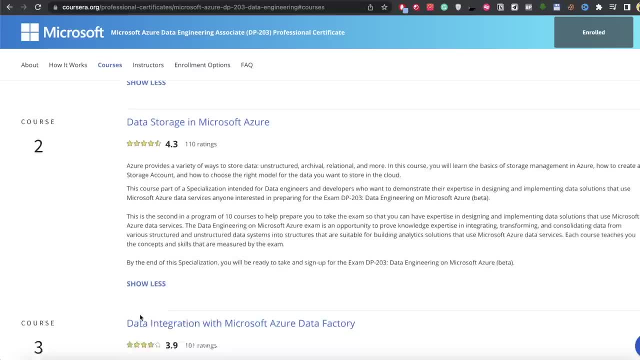 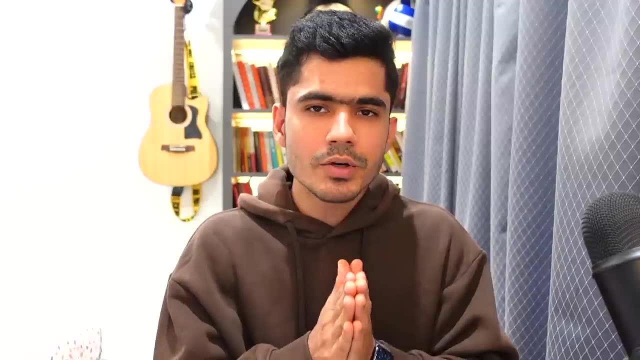 is provided by microsoft itself and will give you the same level of knowledge with the hands-on experience. so you can audit this course for free and if you want hands-on labs and certification you'll have to pay for it. i will put the link of both of these courses in the description now. if 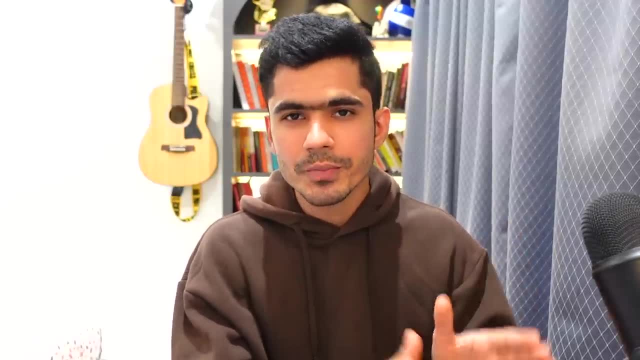 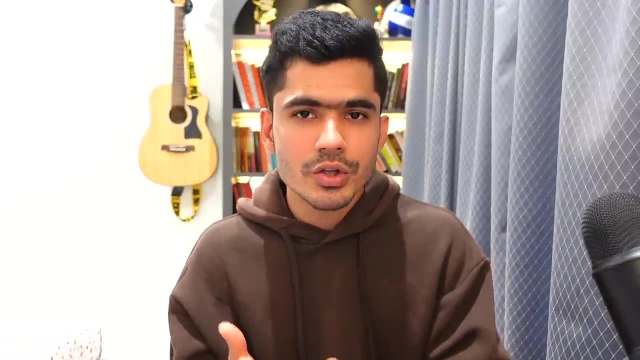 you can't afford any of these courses, then you can also go on youtube and learn from there. there are many amazing series available for free on youtube, so you can just start learning from them and do the hands-on practice along the way while you are watching the video. one of the playlists that i 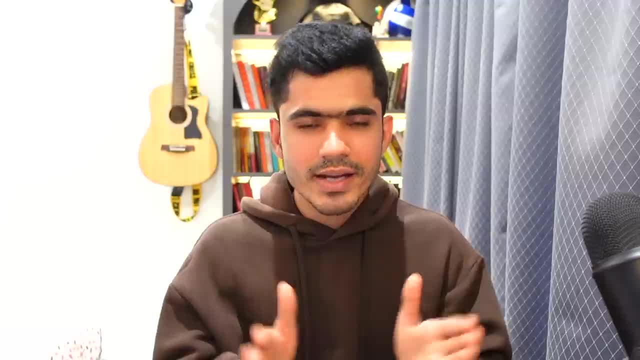 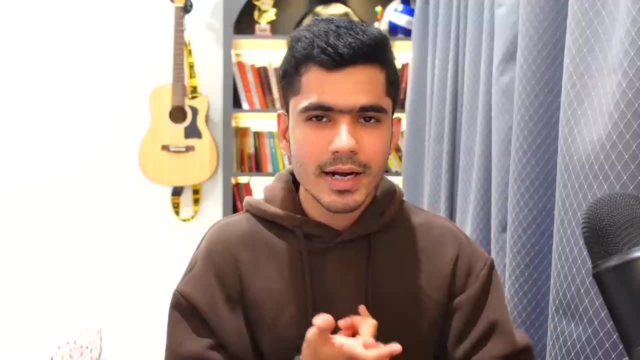 like from the youtube, is this one from the k21 academy. now again, it's up to you. you can pick any of the courses either. you can go with the cloud academy, you can go with the coursera. you can also find some good courses on udemy. i tried to find it, but i could not find any of the good. 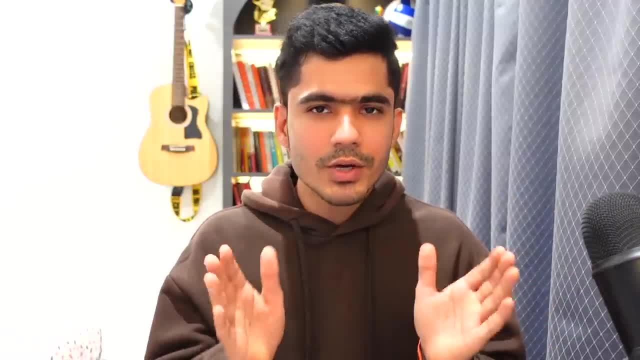 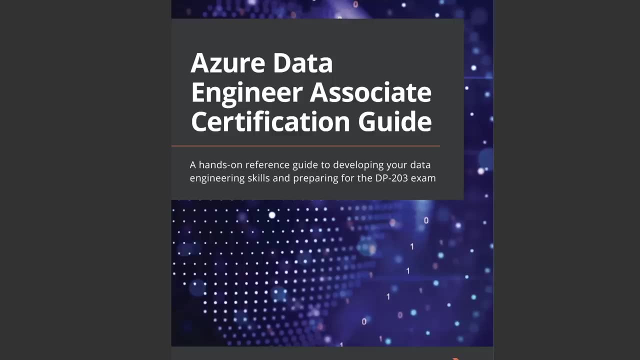 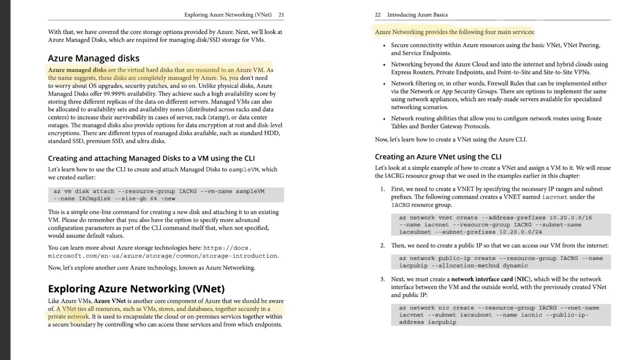 courses, but if not, you can always go back to youtube and learn from there. and while doing the course, i also recommend reading a book. now, this book is one of the best book written on azure data engineering certification. azure data engineering associate certification guide help me to understand different parts of data engineering and how to do data engineering. 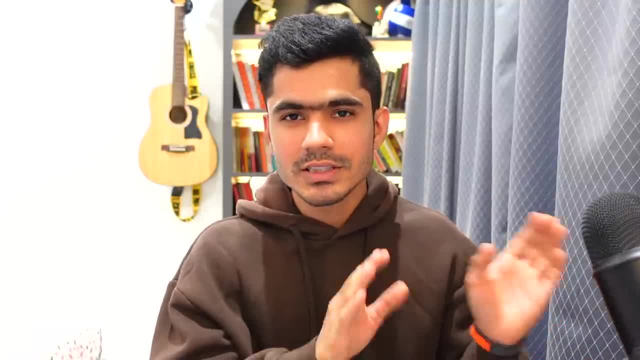 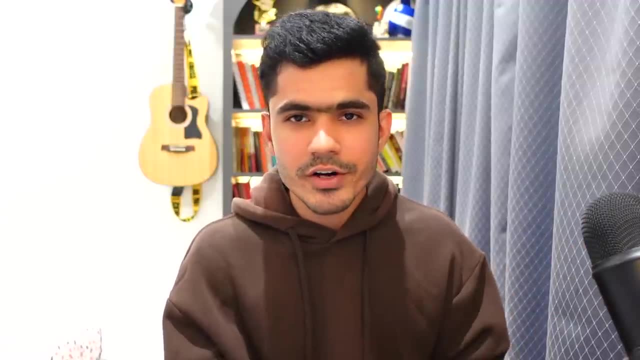 using azure cloud. so whenever i got bored from watching videos, i will start reading this book. that helped me to revise few things and also help me to learn new things along the way. so what you can do, you can start watching the videos if you get bored of it. you can. 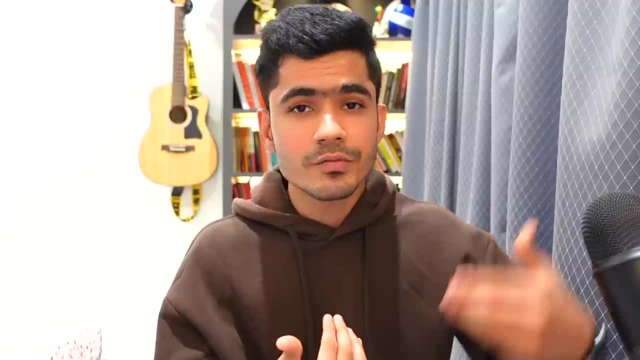 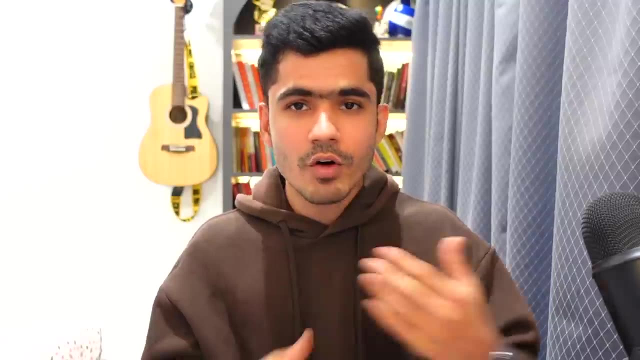 start reading the book. sometimes what happens is that the thing that you learn from the video also is available on the book, so it will help you to revise the things, and sometimes you learn new things from the book. so while watching the videos, if the same topic comes, you will have much better. 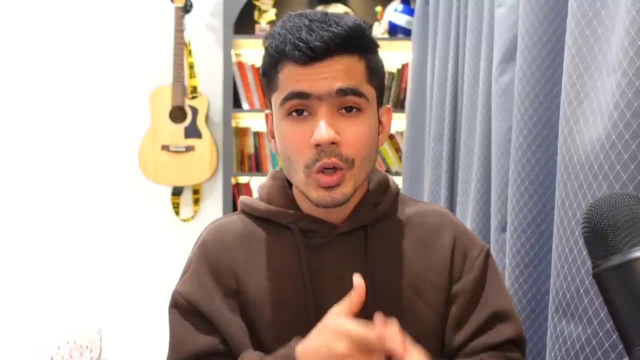 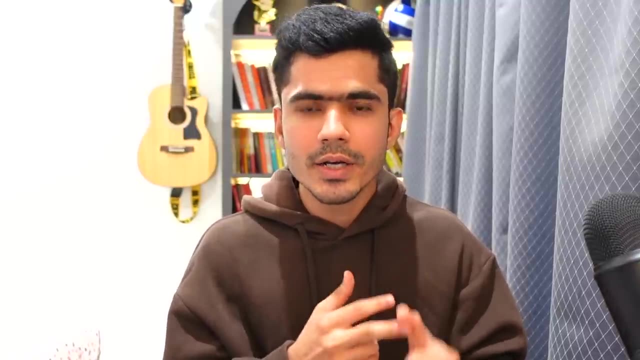 understanding of that topic. so i also recommend reading the book along the way while doing the course. now the third step i recommend is doing the hands-on practice as much as you can. so while reading this book and doing the course, you will get a lot of opportunities to apply all of this. 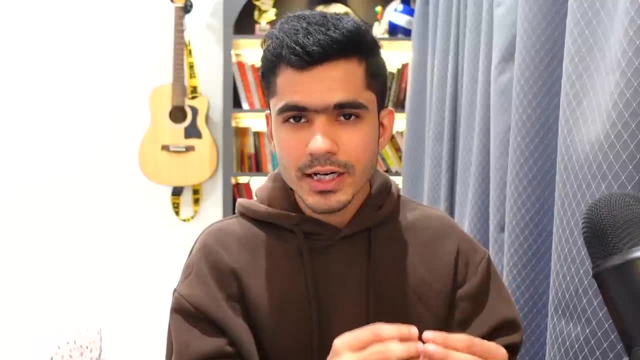 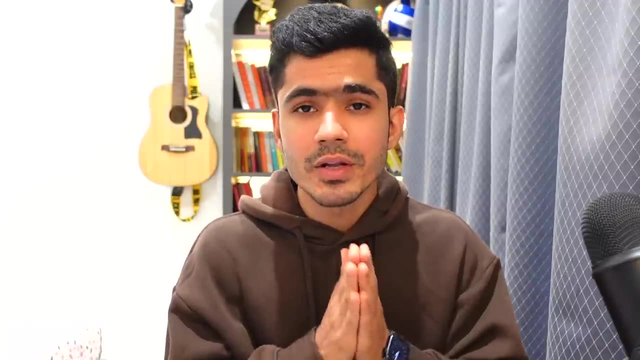 so if you are interested in learning about the azure cloud, you can start doing the hands-on practice by just logging into your azure portal and start implementing them. the more you implement, the better understanding you will get and it will be much more easier for you to answer the. 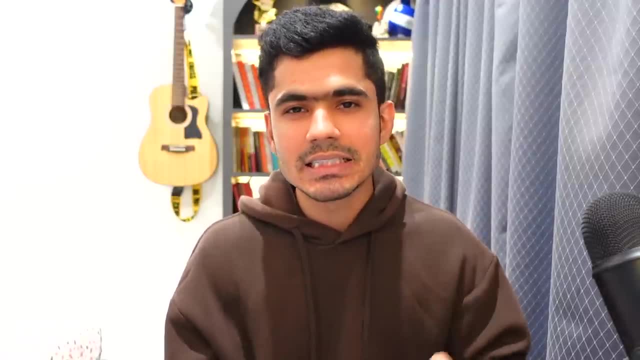 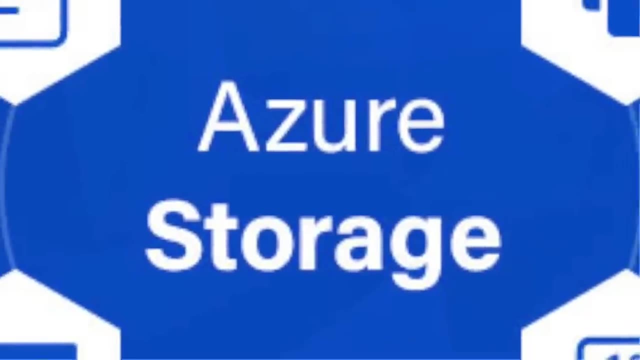 questions in exam. after completing these two steps, you can easily answer 50 of the questions that will come in exam now. here are some of the important services you should focus on. learn about azure storage and different types of it, such as blob, files, tables, queues used for storing various 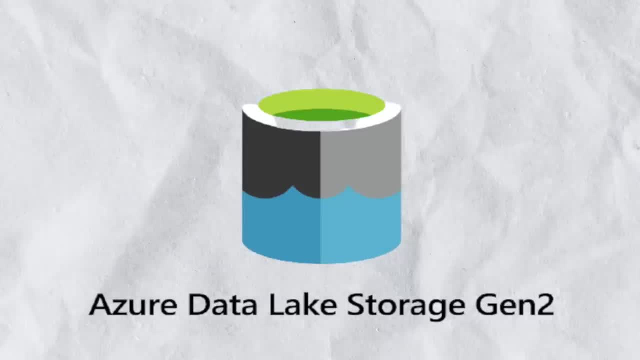 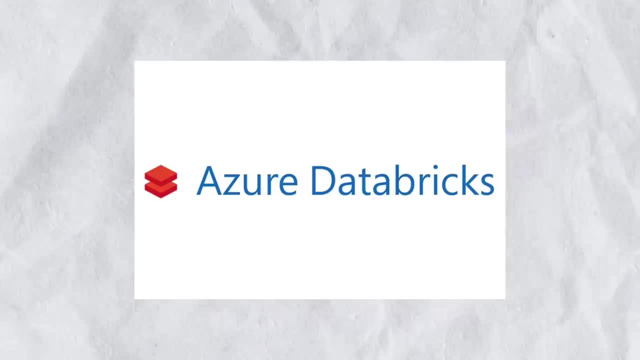 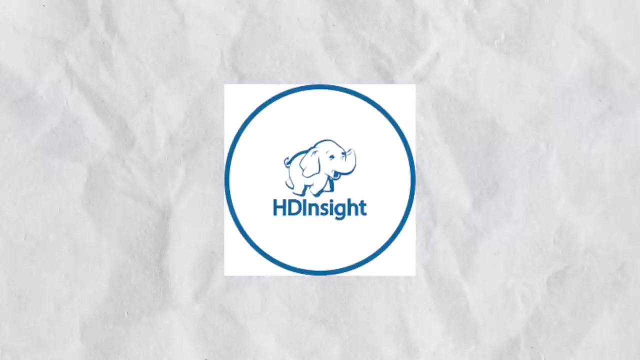 information. azure data lake storage gen 2 used for building data lake data factory to process data and build pipeline synapse. analytics for data analysis and building pipelines database. manage spark environment to write transformation jobs. stream analytics to process real-time data. hd inside open source version of spark hype and hbase cosmos db. no sql solution provided by azure. 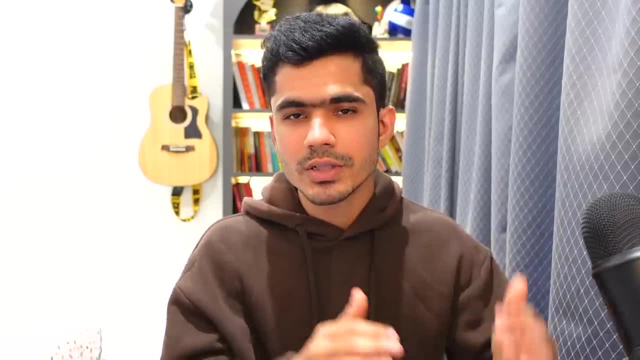 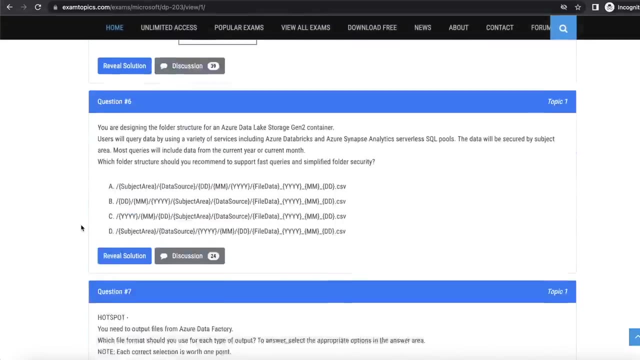 and then there are other few services that you will learn along the way while doing the course and reading the book. now, once you complete all of this, then the last step is to give the practice. for practice exams, i use exam topics. you will get enough questions here for free that will help you. 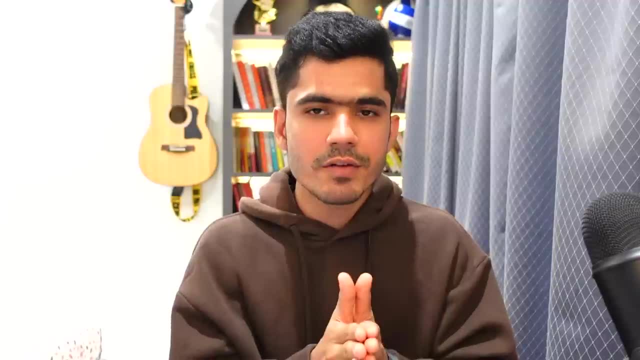 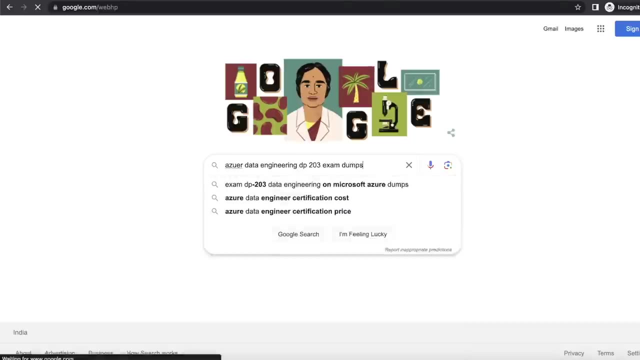 to get familiar with the types of questions that you will face in the exam. the free version of this will give you the limited questions and if you want the complete set, you can pay for it and buy. but you can also just search on google and you will get plenty of exam dumps and resources to. 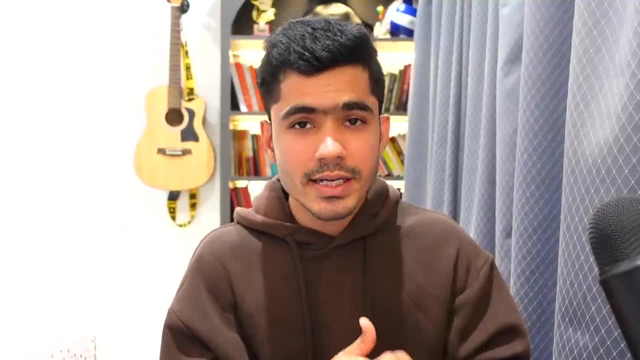 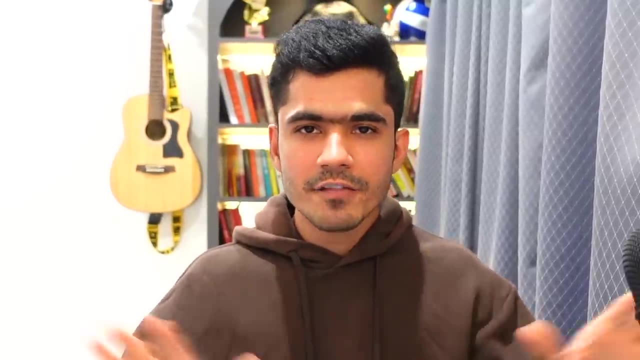 prepare now. here's the thing: i already have the good understanding about data engineering and already worked on aws and gcp, so it was very easy for me to prepare for azure certification because i had the ability to prepare for the exam and i was able to do it within seven days. 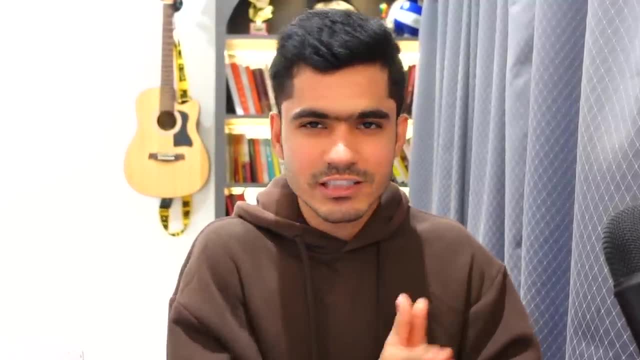 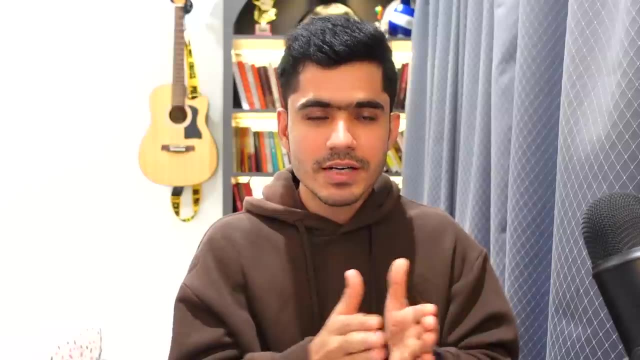 but even if you are a complete beginner, i guarantee you, if you follow this framework, you can easily clear this exam within 30 days. all you have to do is focus on just learning about this. for the seven days that i used to prepare for this exam, i completely forgot everything and just focus on. 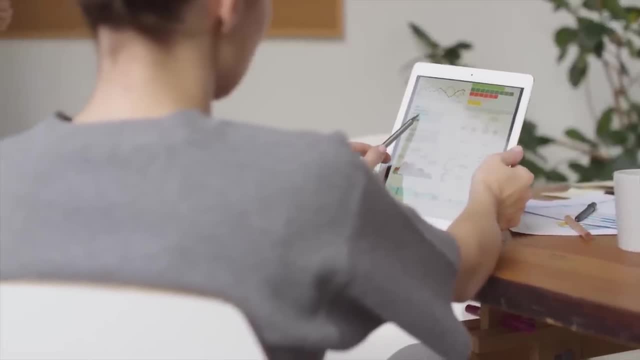 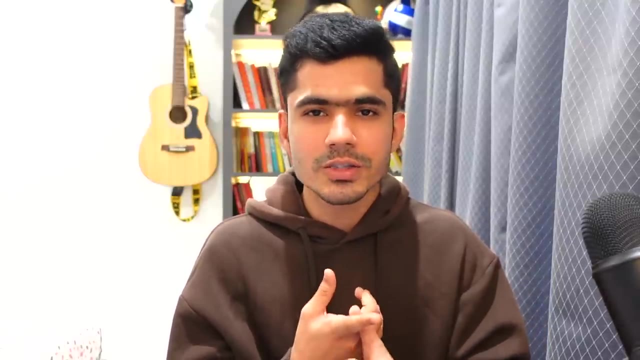 preparing for this exam. you need to get obsessed if you really want to clear this exam. so if you are traveling by train, bus or going out and if you have time, you can start reading from the book. you can start reading from the book and you can also watch some videos online. you need to build your 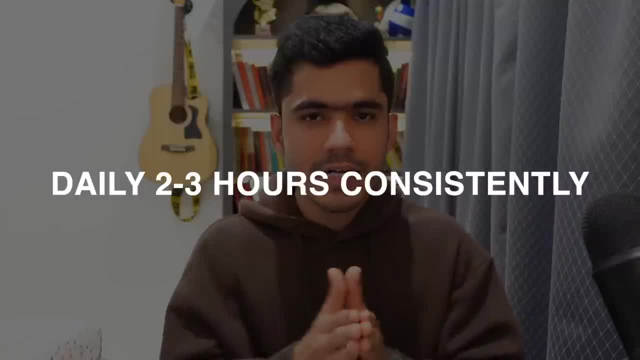 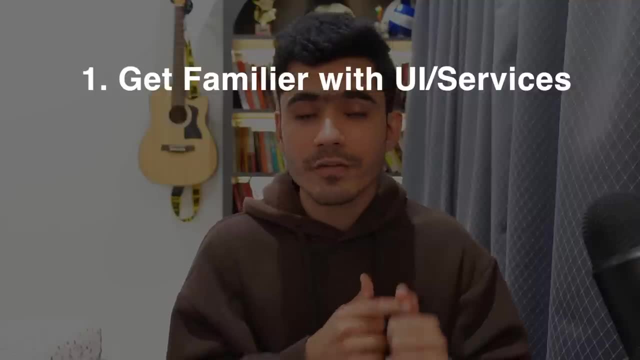 entire routine about clearing this exam. only then and then, you will be able to clear it daily. two to three hours of consistent learning is enough to crack this exam within 30 days. here's the summary. first step is to get familiar with all of the different services and ui, so don't focus on. 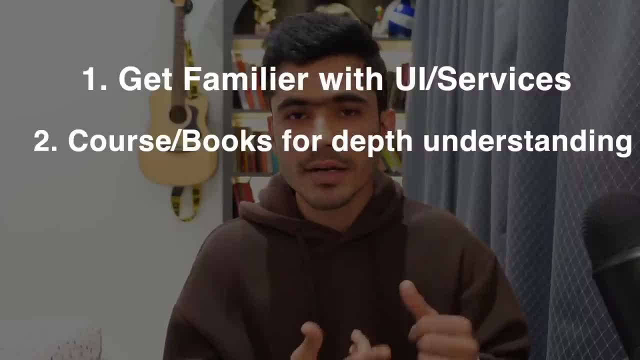 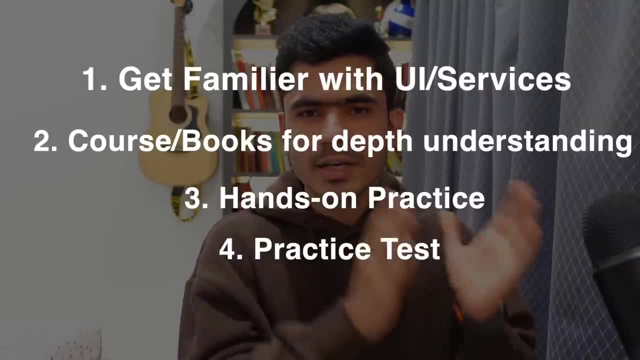 mastering anything. just focus on getting familiar with things and then, in the next step, you can do a course and read from the book, get detailed understanding about all of these things and do the hands-on practice along the way, and once you are comfortable with this, then you can give. 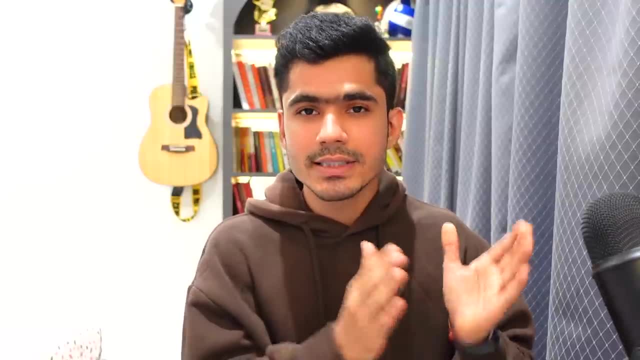 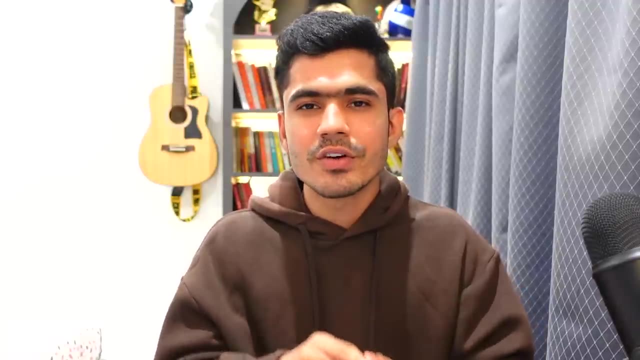 it a try and then appear for the exam at the end. i will highly suggest you to schedule this exam before even you start preparing for it, because you will have the deadline, so you will stay consistent throughout the journey. now, if you watch this video till here, that means you are very 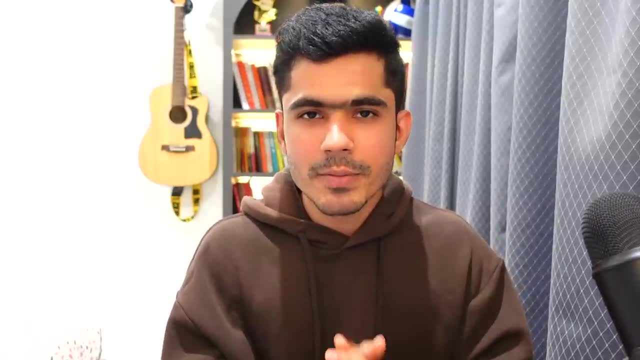 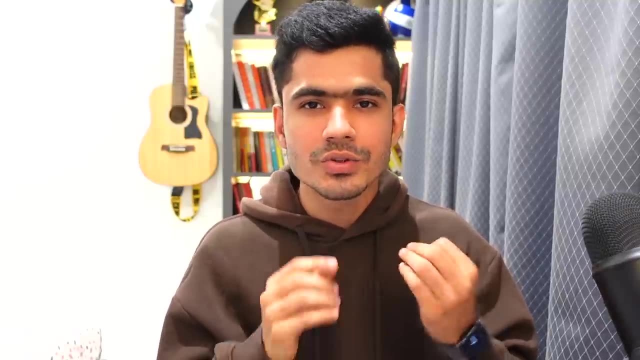 serious about clearing this exam. so what you can do, you can just write the comment below: i will clear this exam in x days, such as i will clear this exam in 15 days. once you do that, then you can come back again after those days and give me the update if you cleared it. if you are still,